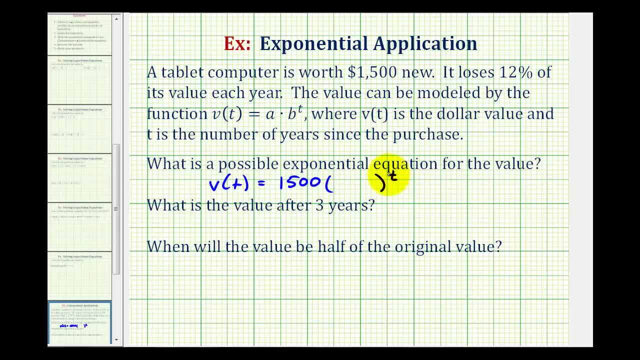 Then we're going to have some base b raised to the power of t. So let's talk about how we're going to find the base of this exponential function. We know, each year the computer loses 12% of the value, which means it retains 88% of the value. 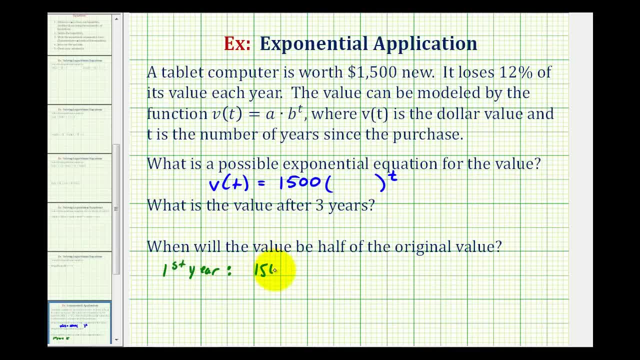 So after the first year the value would be 1,500 times 0.88.. This 0.88 represents the 88% of the value that it retains after the first year. After the second year, the computer loses another 12% of the value. 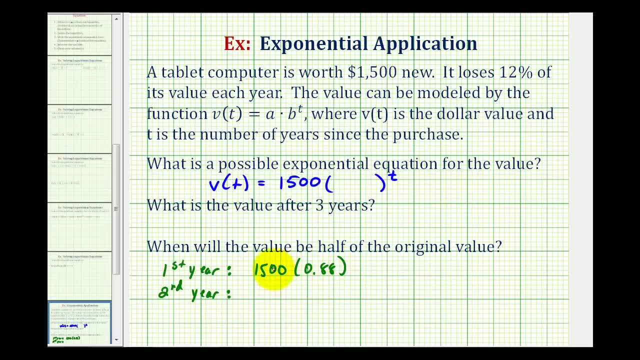 off this amount or retains 88% of this value here. So after the second year it would be 1,500 times 0.88, times another 0.88.. Again, the second 0.88 represents the amount of value retained after the second year. 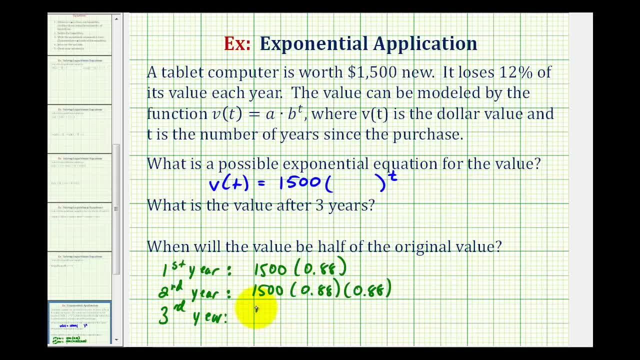 and this pattern is going to continue After the third year, we'll have 1,500 times 0.88 times 0.88 times another 0.88.. So the base of our exponential function is going to be 0.88,. 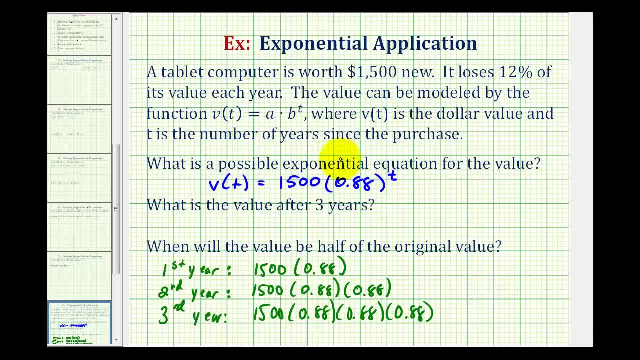 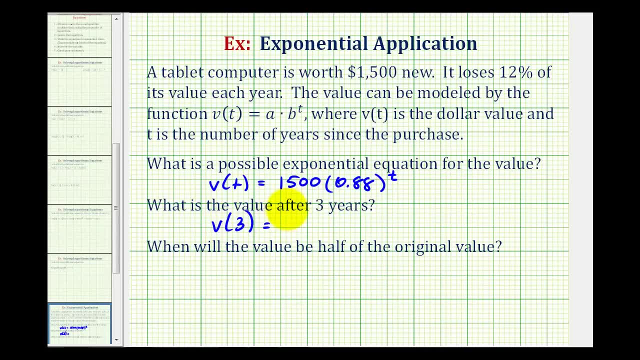 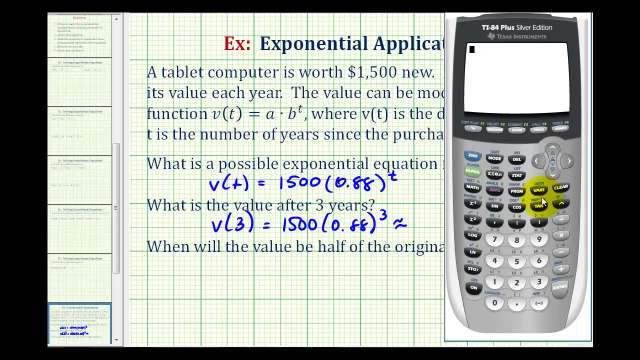 which is the percent of value the computer retains after each year. So to find the value after three years we need to determine v of three. so we'll substitute three for t and evaluate this on the calculator. So we'll have 1,500 times 0.88. 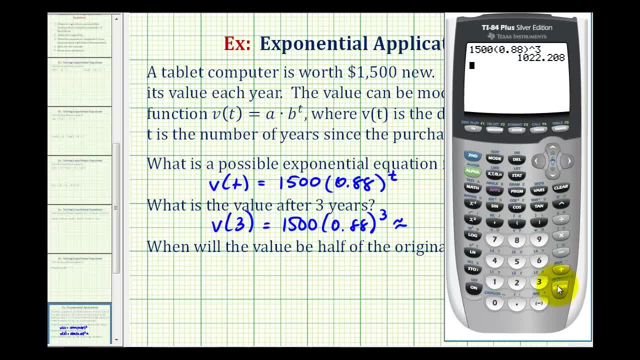 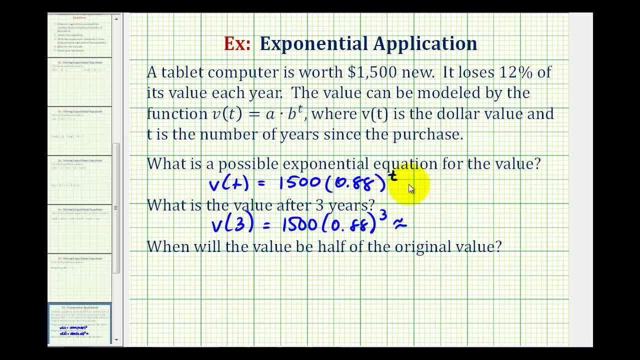 raised to the power of three. So the value of the computer is approximately $1,022.21 after three years. And now for the last question: when will the value be half of its original value? Well, the starting value is 1,500,. 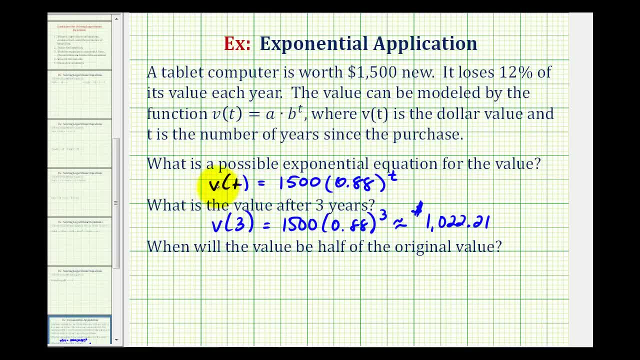 so half of this would be 750.. So we want to set v of t to 750 and then solve for t. So we'll have 750 equals 1,500 times 0.88 raised to the power of t. So we want to isolate the exponential power.